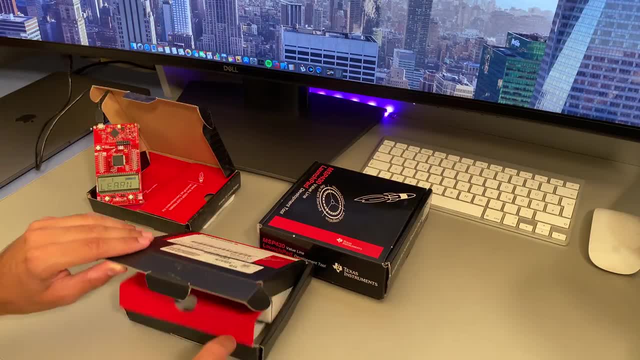 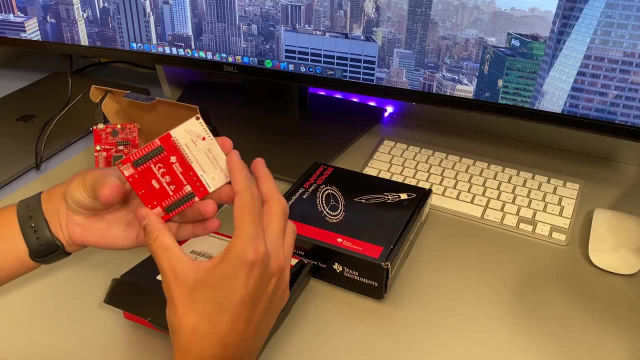 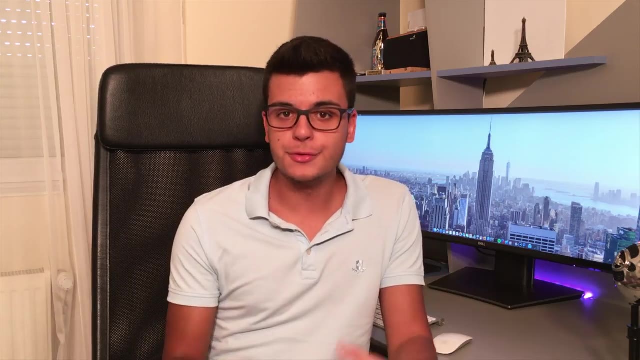 selection of microcontrollers. it has a great community online and also Texas Instruments offers a lot of documentation and great examples for each and every microcontroller and each and every peripheral that microcontroller has. This includes code examples and also documentation. Now we are going to talk about the 5 peripherals you need to understand if you want to start. 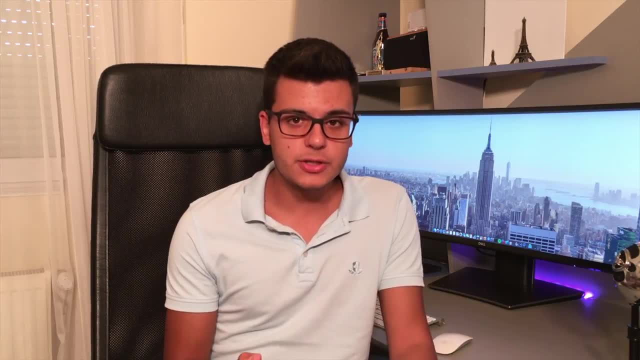 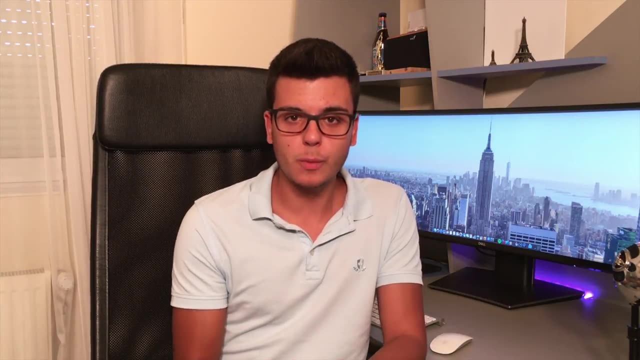 learning embedded systems. I am not going to into formulas or implemntations. I am just going to explain to you what each and every one of these peripherals does and how they can be useful if you nämlich want to build an application. The first peripheral we are going to talk about is GPIO, or general. 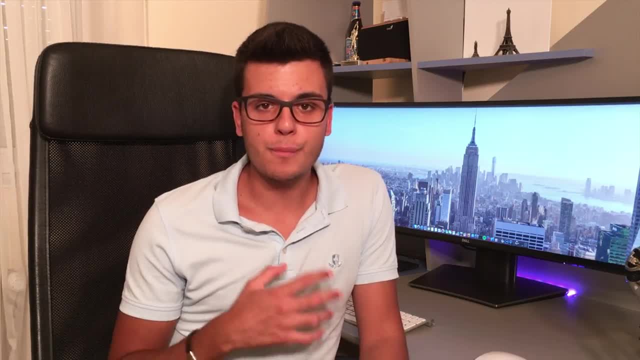 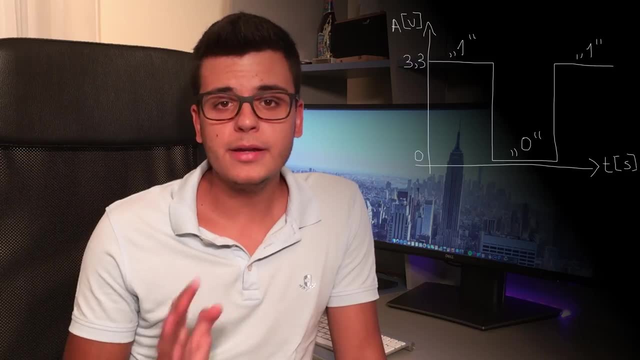 purpose- input, output- and these are basically ways for your microcontroller to connect to the outer world, Basically just like ports on your computer, but they're much simpler. They can either output one of two values or read one of two of the same values, and these values are logical zero, which 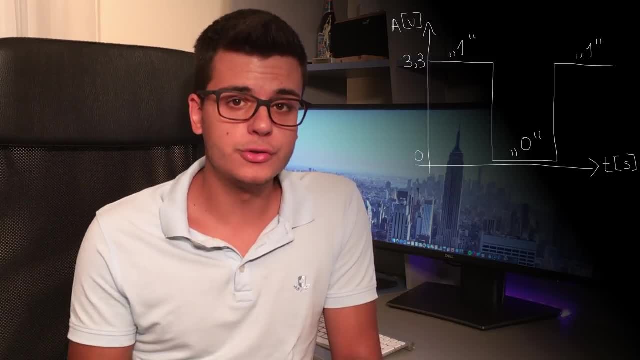 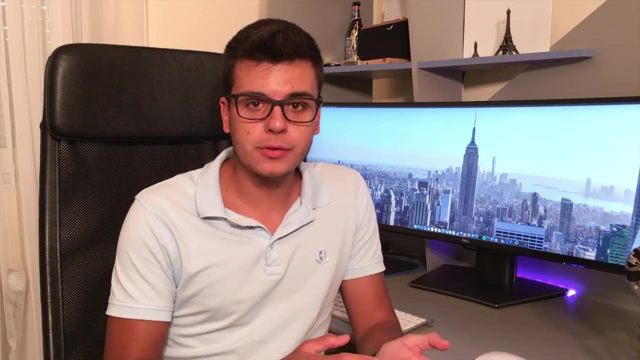 corresponds to zero volts, and logical one which corresponds to usually about three to five volts, which is basically the supply voltage of the microcontroller. The way you would read or output a value to and from a port which is basically just a physical pin is through registers and 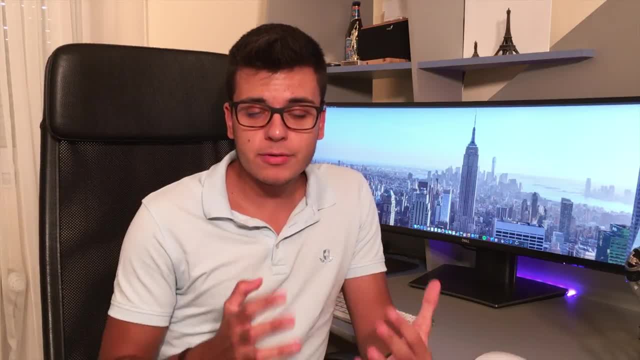 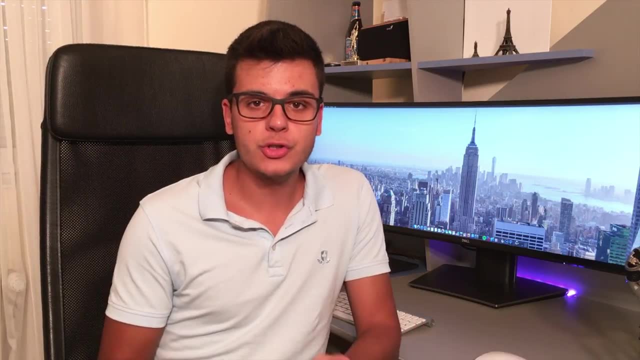 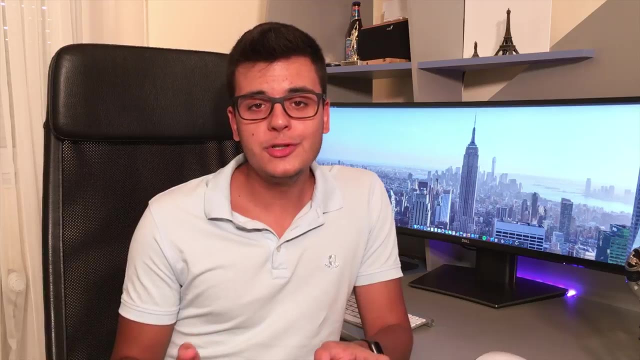 registers are really important if you want to understand peripherals, because every time you're going to work with peripherals, you're basically going to work with their registers. All that registers are is location memories which are allocated to a specific peripheral so that you can actually interact with it, set it up and take values from it. So how would GPIO be useful in a 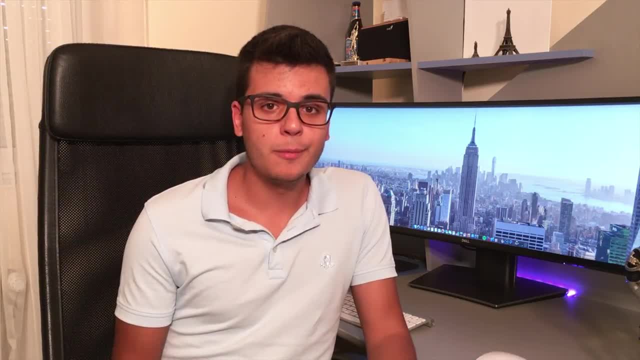 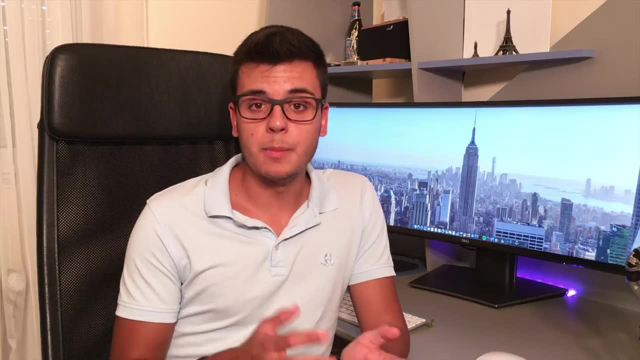 application. Well, there's a lot of things that you can use these for, but some simple examples could be to turn on or off an LED, or to signal to another system the fact that a process went through without an issue or that you have errors. So you would basically output logical one if that. 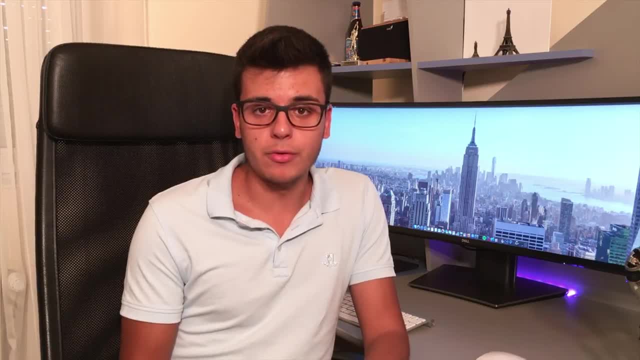 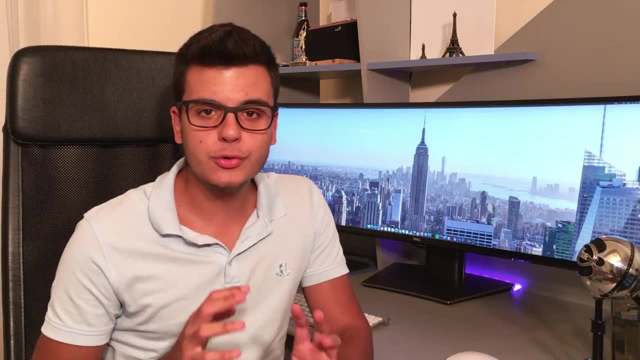 process didn't have an error, or logical zero if there were errors within the process. The second concept we are going to talk about is going to be interrupts, and these come in handy when you're trying to run a block of code right after an event happens- Unlike polling, which means 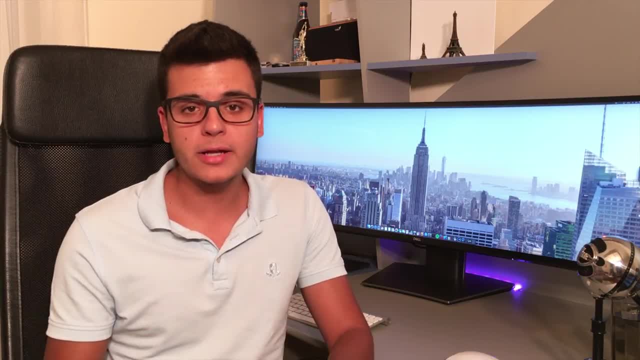 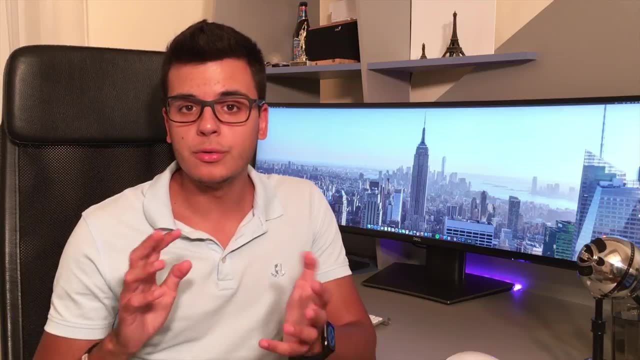 you have to wait inside the loop for a condition to be met or for a flag to be set with interrupts. all you have to do is write an interrupt handler, which you can think of as a function that gets called right after an event happens, So you're not wasting CPU cycles just waiting for an event. 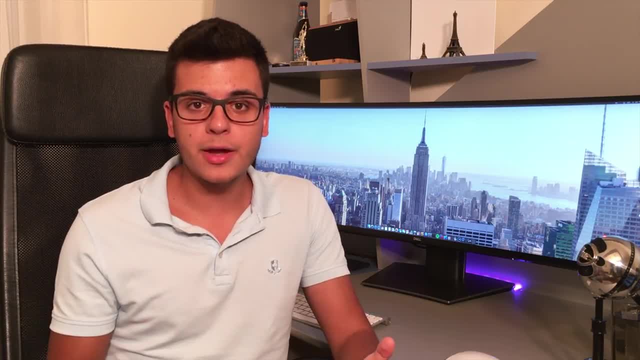 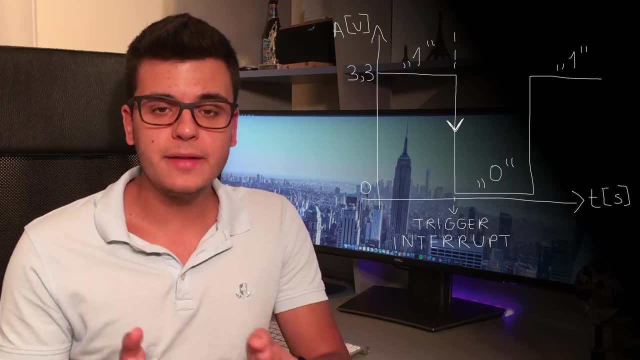 to happen. All you have to do is set the event which will trigger the interrupt, and then you can go on and execute other code until the event happens. As you can see in the figure that I've drawn, I've set the falling edge of that signal to be the source for the interrupt. So if you're 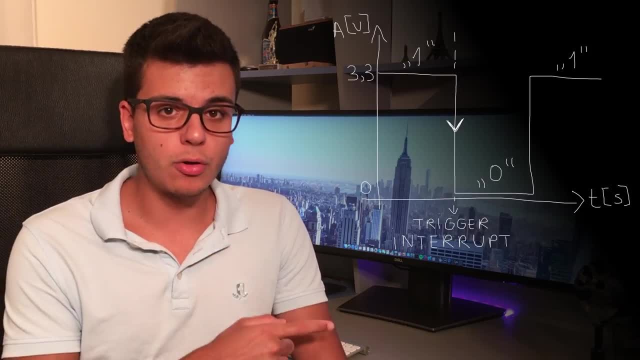 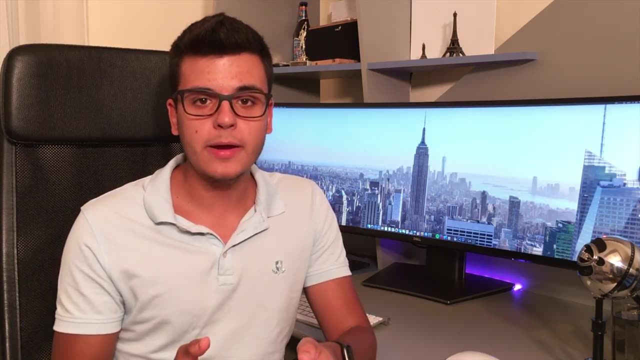 going to run a block of code and you have an error on that signal. you're going to have an error on that physical pin. basically, The interrupt is going to get triggered Again. in this example, it implies that you're going to supply a signal to a physical pin, to the microcontroller, but this 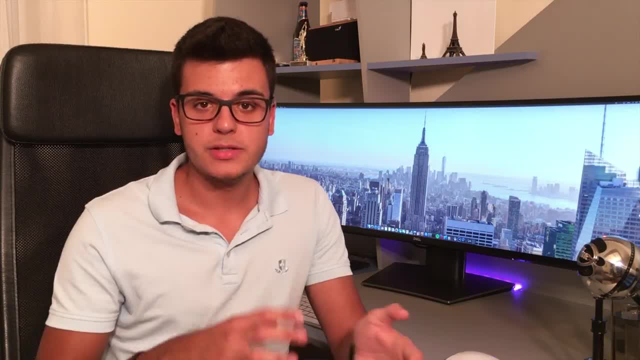 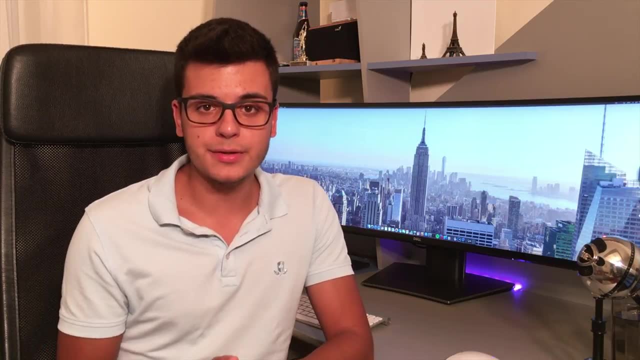 doesn't necessarily have to be a signal. It can be something internal, such as from another peripheral. Maybe it finished a process, or maybe it's thrown an error or something like that. It can really be a lot of things. The third peripheral we are going to talk about is going to be the 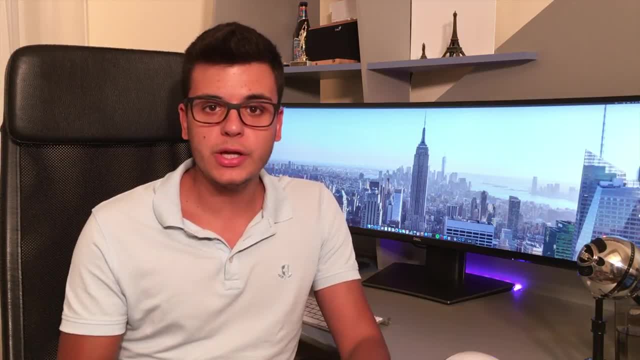 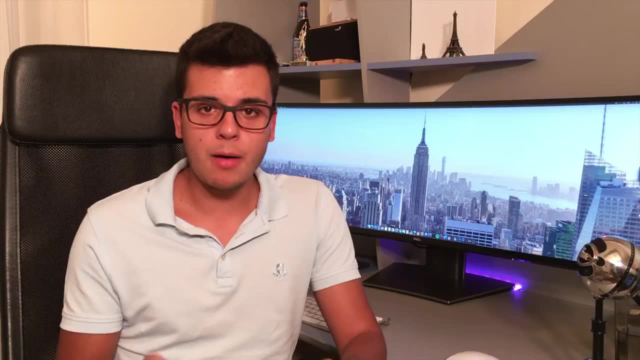 timer, And so with the timer, you can create a lot of things. You can create a lot of things: timeouts, you can count how long a process takes, or you can even create a real-time clock. So a timer usually counts up, up and down, or continuously, and what counting up means is that you actually set. 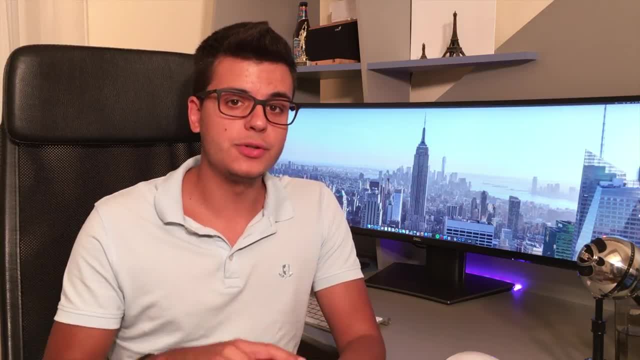 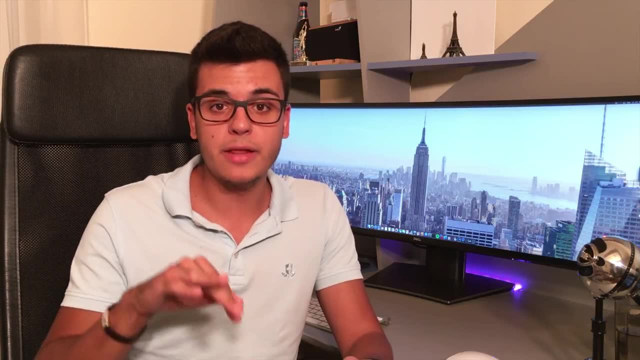 a value in the register and the timer counts up to that value and when it reaches that value, it starts over from zero. Count up and down, on the other hand, means that your timer is going to count up to that value that you just set and then it's going to start counting back down to zero and then. it's going to start all over And with count continuously. it doesn't matter which value you set. the timer is going to count until it overflows, so it reaches its maximum value and then it starts again from zero. The maximum value a timer can count up to is going to be dependent on how many bits the timer is actually running on. 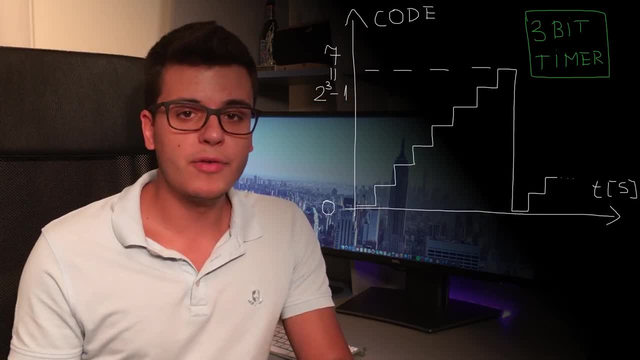 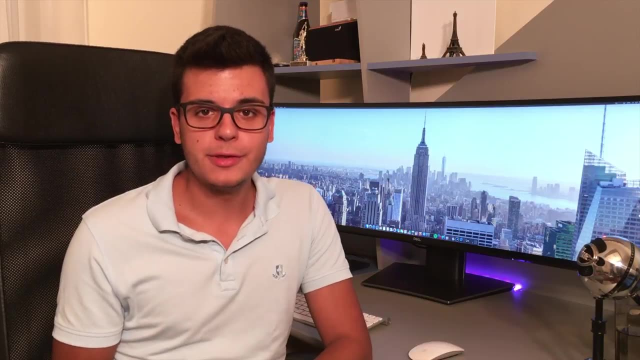 Just for example, if we have a 3-bit timer, the maximum value it can count up to is going to be 7.. So this means 2 to the power of 3 minus 1.. Usually, timers nowadays also includes modules named CCP. 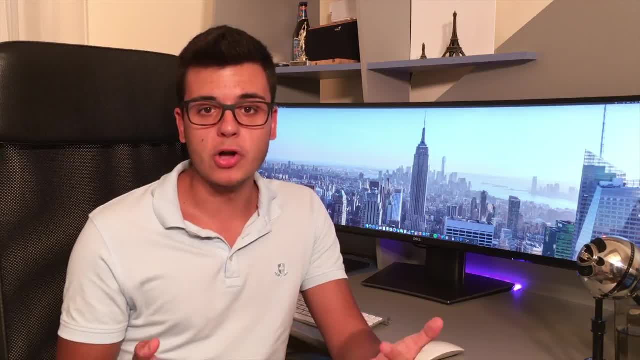 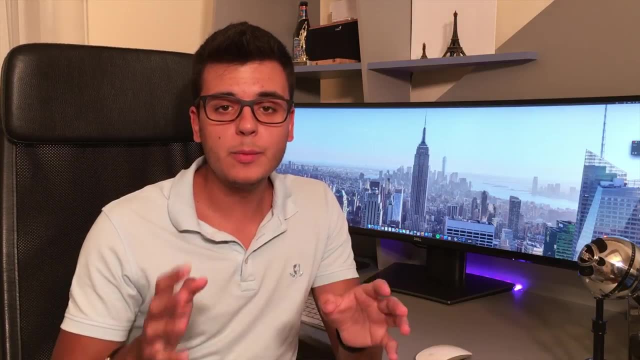 Or capture, compare and pulse width modulation modules. The capture mode allows us to time different processes, and the way we do this is by supplying a signal to the module, and then we can actually find a time difference between two edges of that signal. This happens by saving a snapshot. 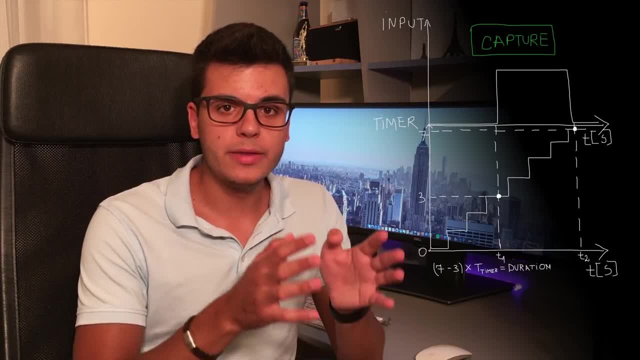 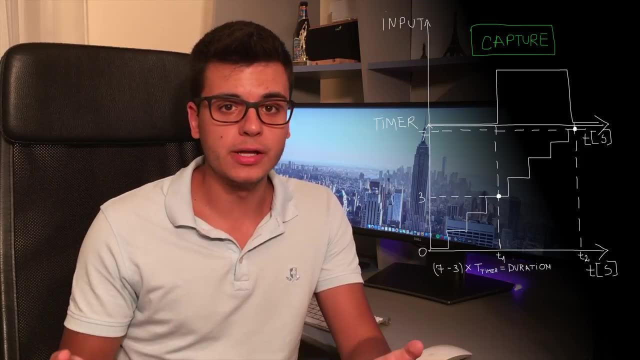 of the value that the timer has counted up to when the edge happened and then when the other edge happened, And then it's just a matter of subtracting these two values and just converting it into time, because we know the frequency with which the timer is going to be running. So if we have a 3-bit timer, 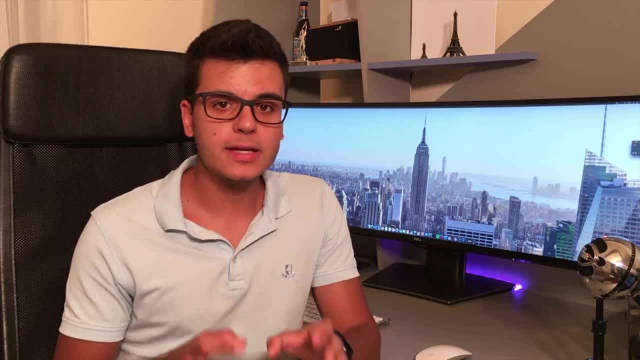 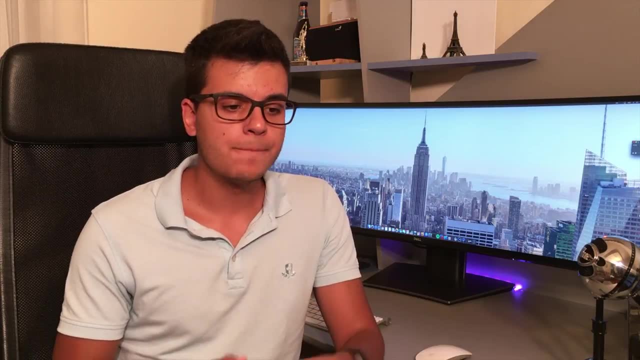 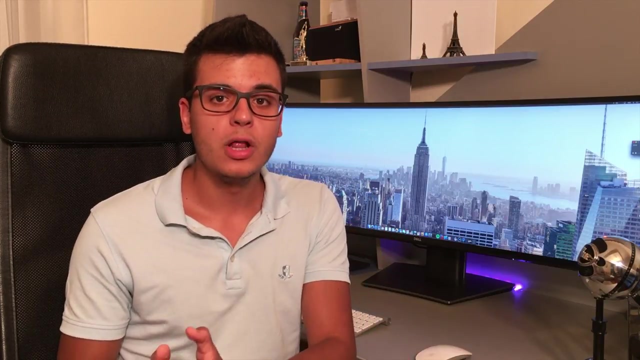 it counts up. The compare mode is kind of the opposite, because it allows us to output pulse width modulated signals or signals where we modify the duty factor. So we have a fixed frequency and then we can choose how long the logical 1 or logical 0 lasts within one period. This would, for example, 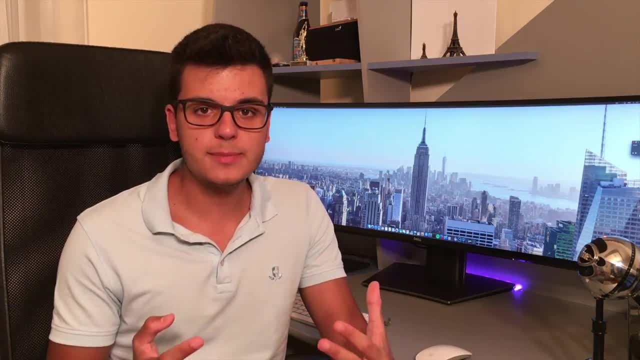 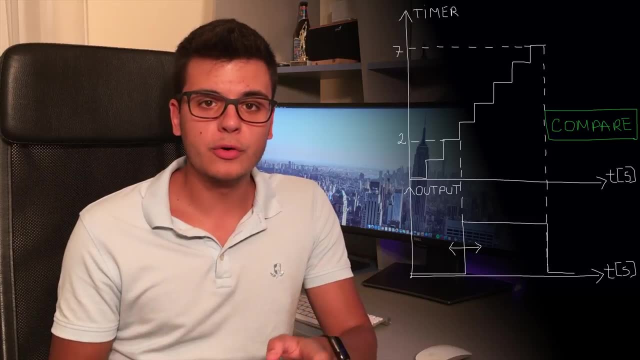 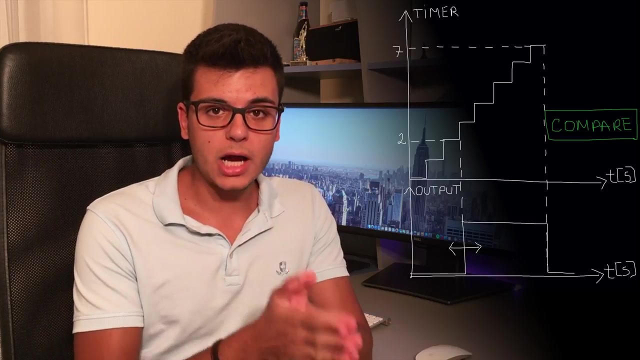 be useful if we want to control how fast a fan spins, which is basically a DC motor, or if we want to control how much light an LED outputs. The way the compare mode works is by setting a value in a register and then the timer is going to create an edge on the output signal when the timer counts up to that value, and then the other edge happens when the timer overflows. 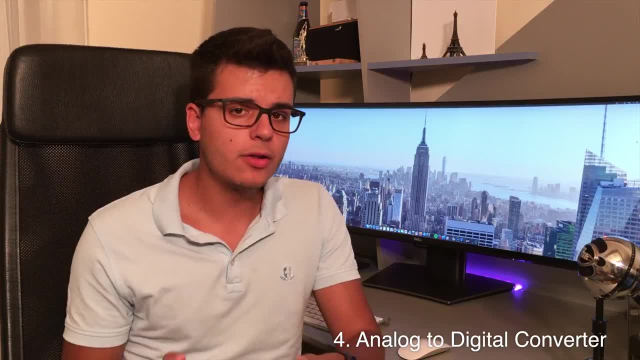 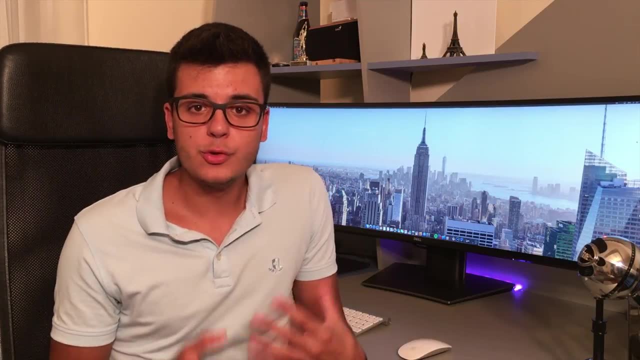 The fourth peripheral is going to be the ADC, or the analog to digital converter, and what this allows us to do is to actually work with analog inputs. So if you have a voltage that you want to measure, you can use this to actually get a number you can work with in software. 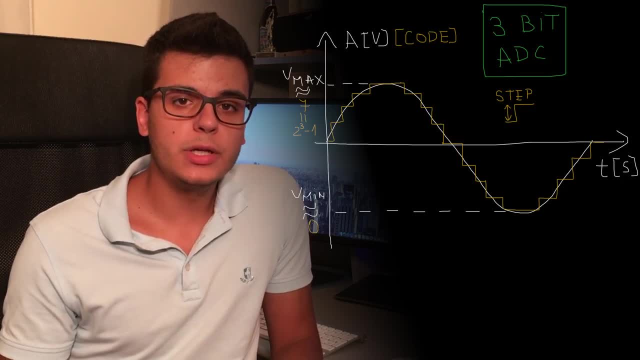 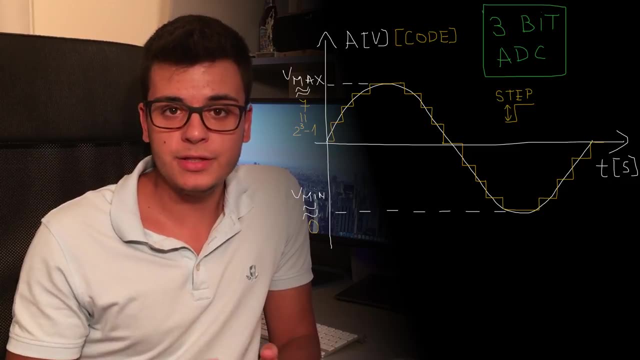 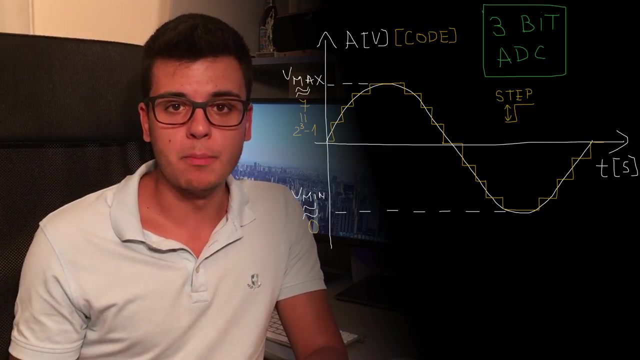 As you can see in the figure, though, this only works between two boundaries, and so you would have a minimum and a maximum voltage, and this is because you actually need to have these voltages as references, and you can't surpass them. You can also probably notice that this peripheral only outputs integer numbers. 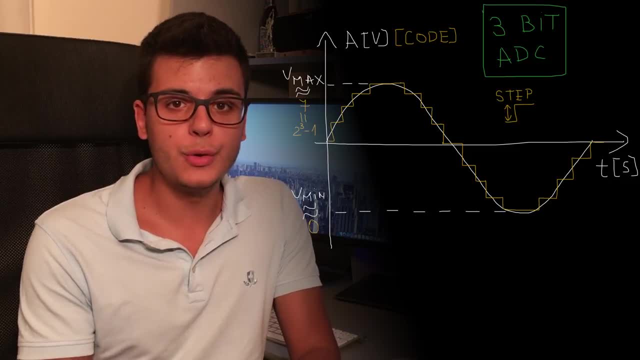 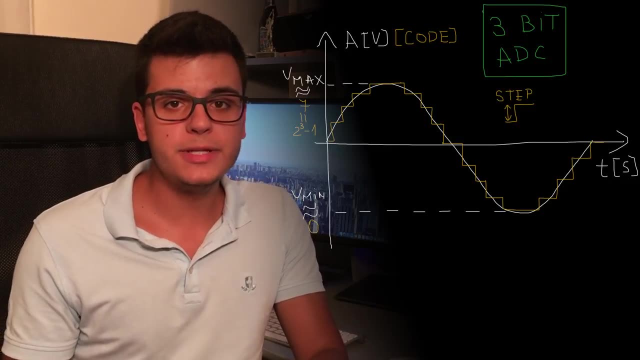 This means that there's going to be an error between the value that you're going to input to the peripheral and the value that you get as an output. This is referred to as the quantization error, and it's always going to be smaller than half of the quantization step. 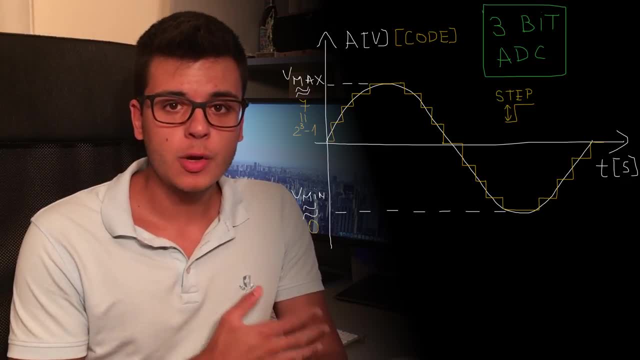 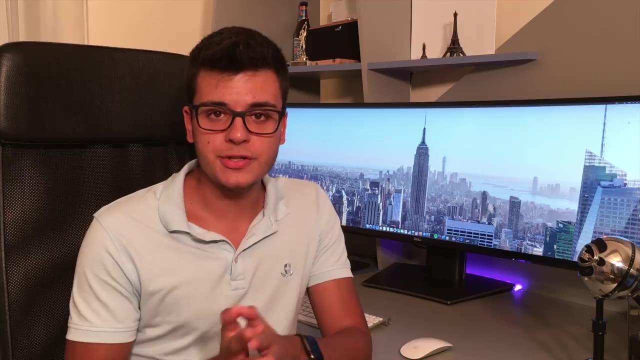 Again with a 3-bit ADC. as you can see in the figure, we have eight steps, from 0 to 7, and these are going to be your outputs. There's also the opposite of the ADC, which is a DAC, or digital to analog converter, and not as many microcontrollers have this peripheral. 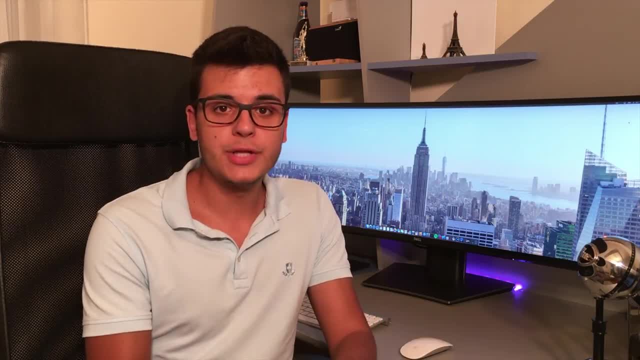 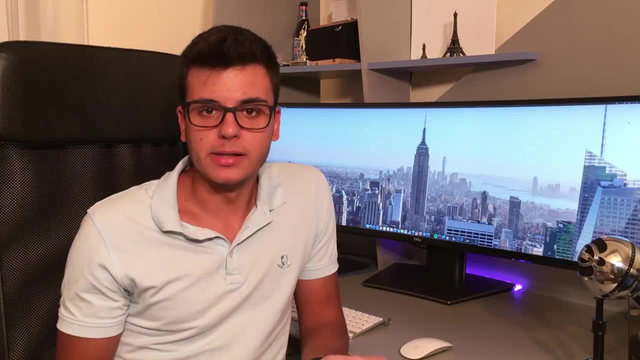 but it's useful if you want to output a signal from values that you have stored in your memory. The fifth and final peripheral we are going to talk about is going to be serial interfaces, and these basically allow us to transmit data to other parts of our system, or even to other systems. 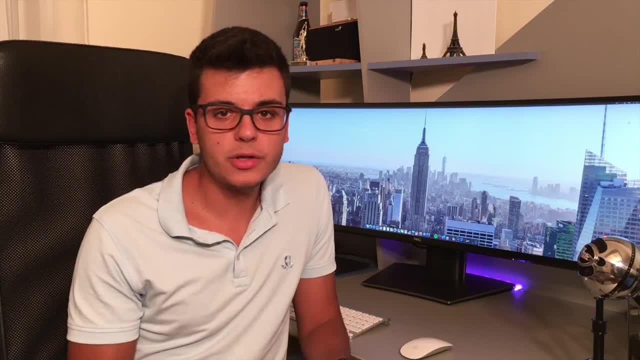 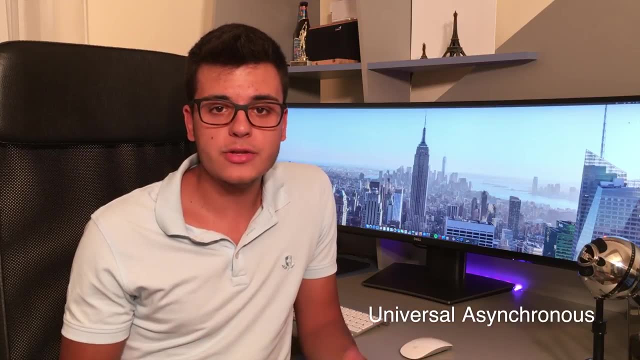 Today I'm going to talk about the three most basic ones, but there's actually quite a lot of them out there. The most basic one is going to be WART, which stands for Universal Asynchronous Receiver Transmitter, and it only requires two data lines. 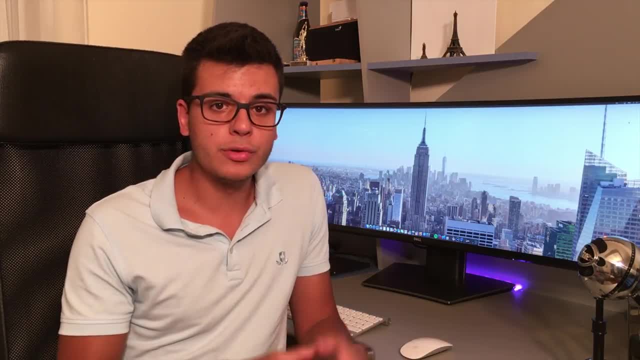 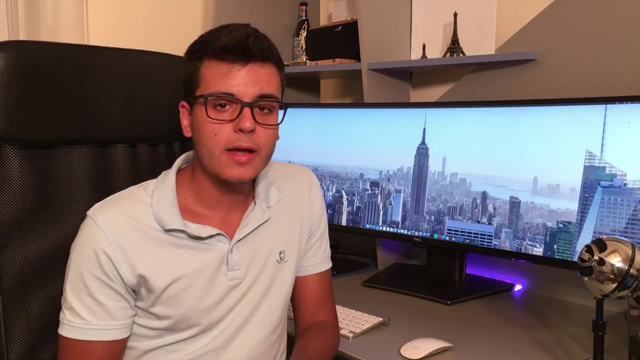 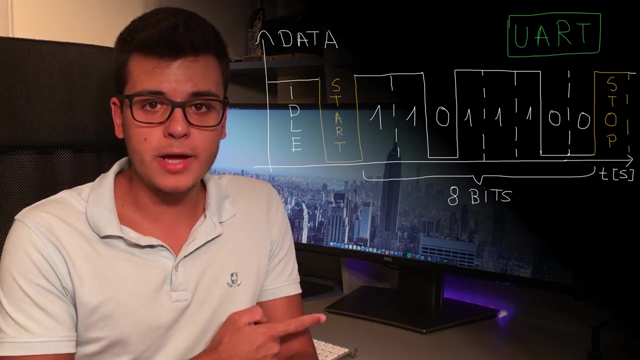 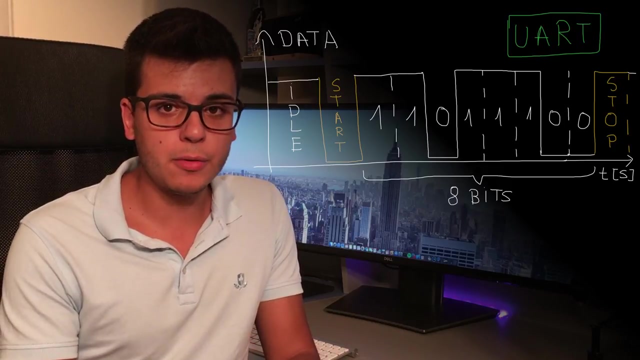 Though simple, it requires setting up the baud rate, or the rate at which you're transmitting data on both systems which are going to communicate, before actually initiating the communication, and it also doesn't allow more than two devices to communicate at once. As you can see in the explanation figure to my right, you basically have a start bit followed by 7 to 8 data bits, one parity bit, if this is enabled, and then a stop bit. 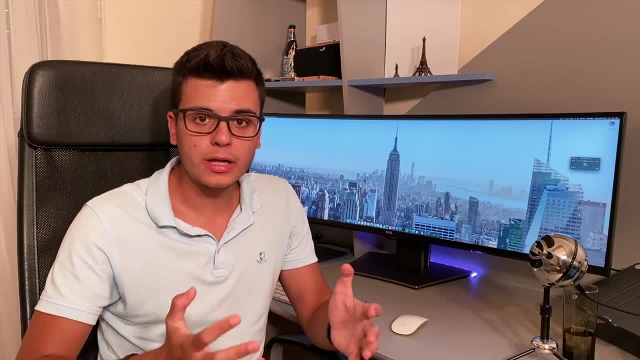 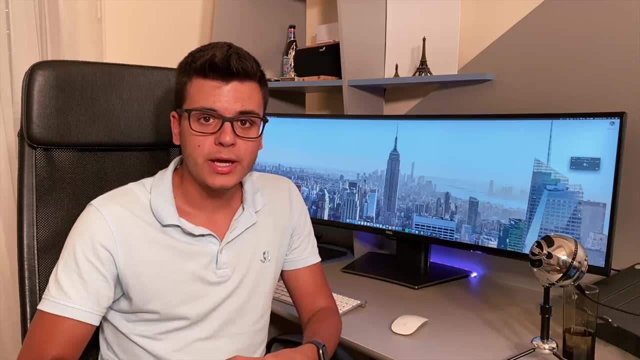 In contrast to WART, SPI and I2C both allow for multiple devices to be connected to the bus and for faster speeds. So SPI is the fastest out of the bunch. it has two data lines and one clock line, which you can think of as a synchronization line. 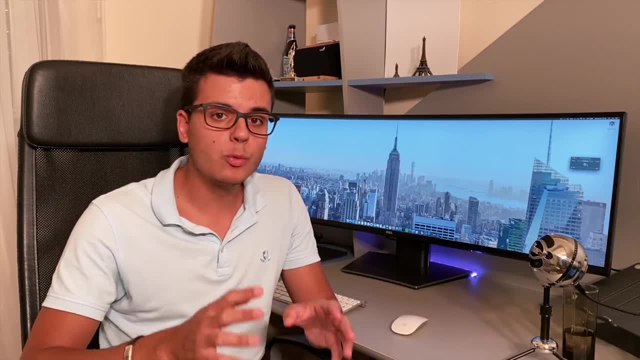 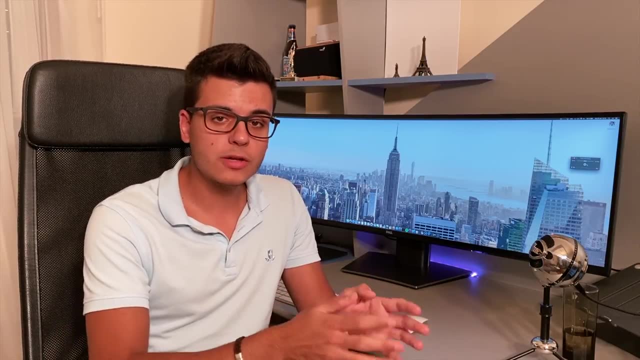 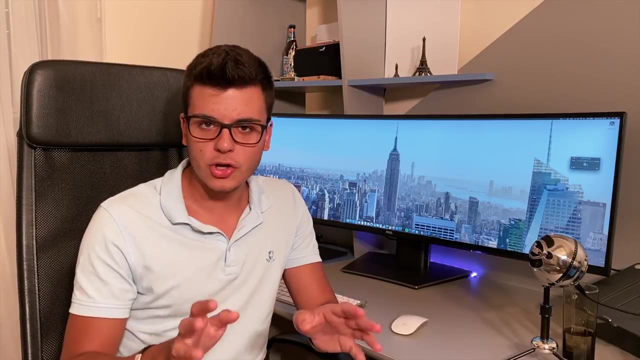 and the way you talk to multiple devices is by having one clock line. You have a physical pin connected to each and every one of them, so another line which just selects which device you're talking to. The way you select a device is usually by outputting a low voltage to that pin. so logical zero. 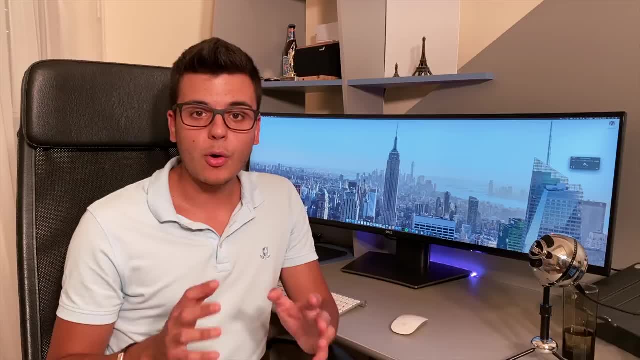 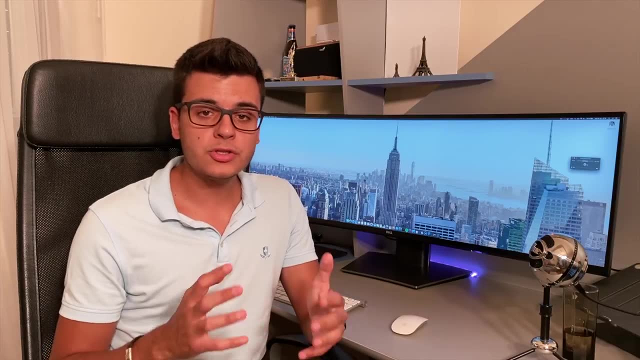 I2C, on the other hand, is slower than SPI but only has two lines in total. so one is for data and the other one is for clock, And the way you actually select which device you're talking to is through an address. So, before actually sending data, you're going to send the data line. 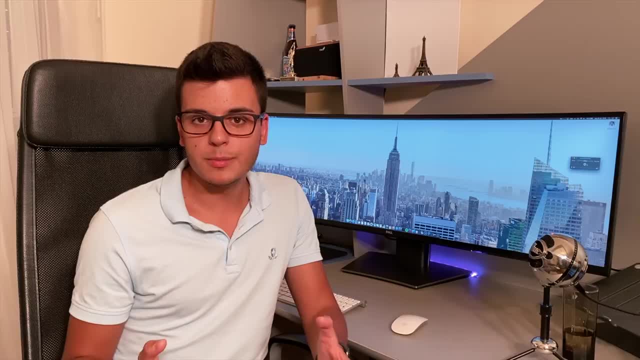 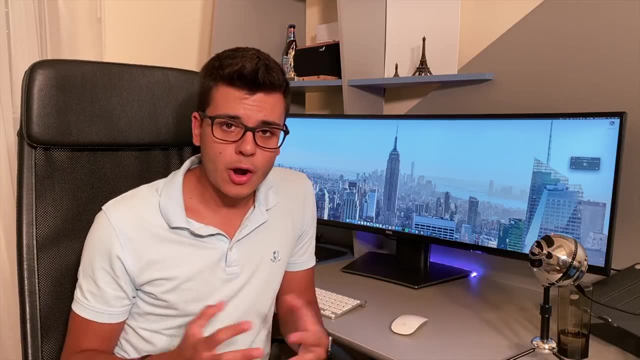 You're going to send the address of the device you want to talk to. This, of course, implies that each and every device is going to have a unique address on this bus. Wow, this turned out to be longer than I thought, but I hope it was helpful for you. 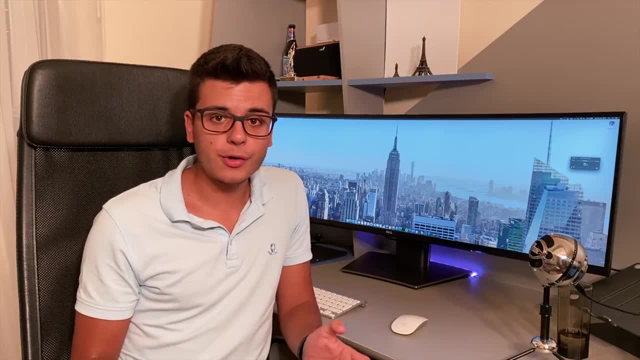 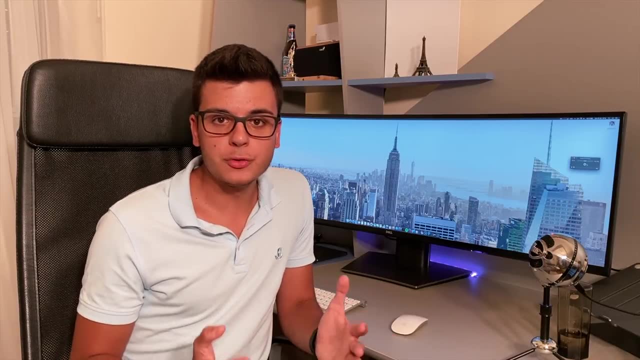 And just so you know, there's a lot of things under the hood that are going on that you're going to learn eventually. But at first, if you understood or are going to understand these concepts, it's going to be enough to start programming easy applications. 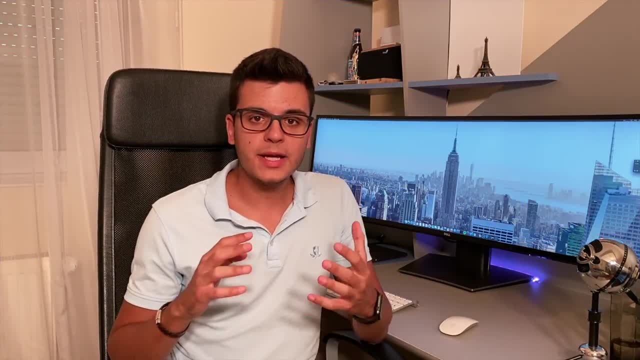 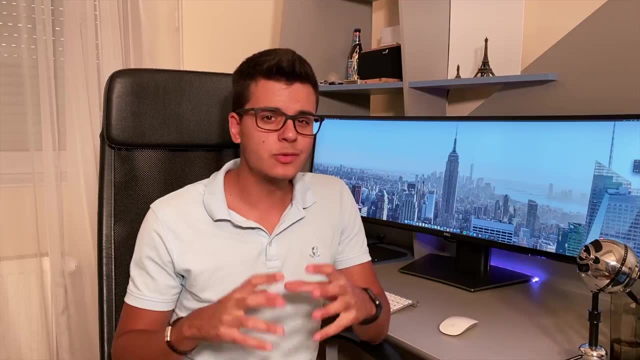 The reason why I don't actually recommend Arduino for beginners is because it has so many layers- So many layers of software on top of the hardware- that you're not really actually interacting with the hardware, And that's what's most exciting when you're going to work with embedded systems. 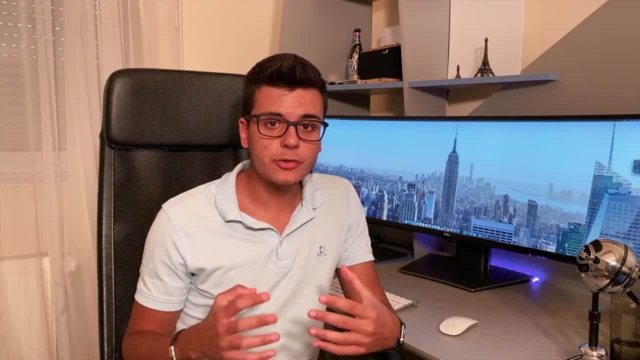 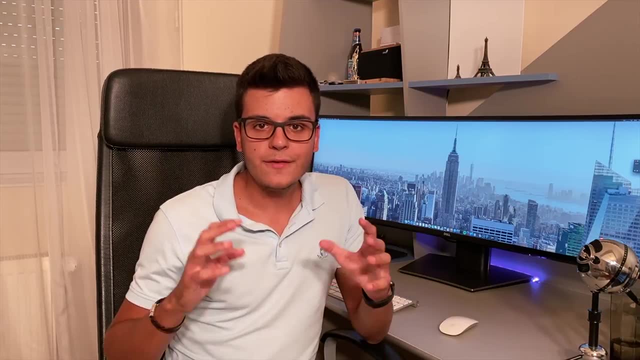 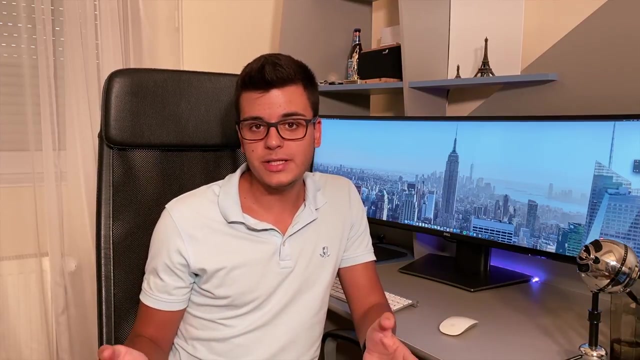 Later on, when you understand all of these concepts and you just want to code a quick and dirty prototype, you're going to be able to use Arduino, But in the beginning it's just really not worth it. If you want to see more videos on topics like this one, make sure to like this video and tell me in the comment section down below what actual topic you want to see me make a video on.